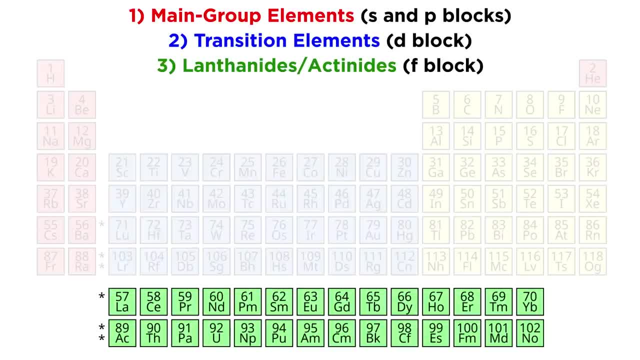 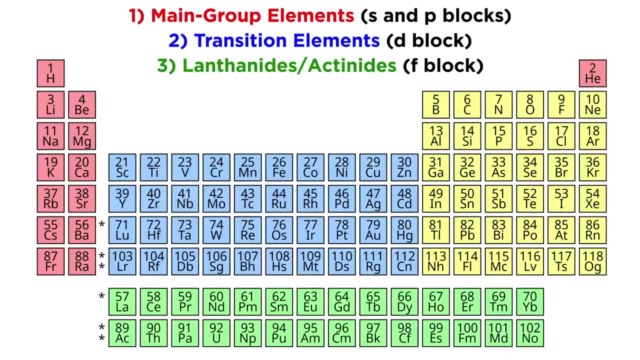 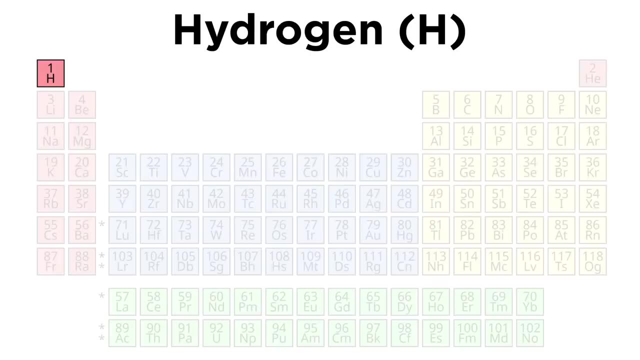 D block or transition elements, followed by the F block or the lanthanides and actinides. But before we cover any of these, we are going to start out by discussing one little misfit of an element. We will spend this tutorial talking about hydrogen. Hydrogen will be covered on its 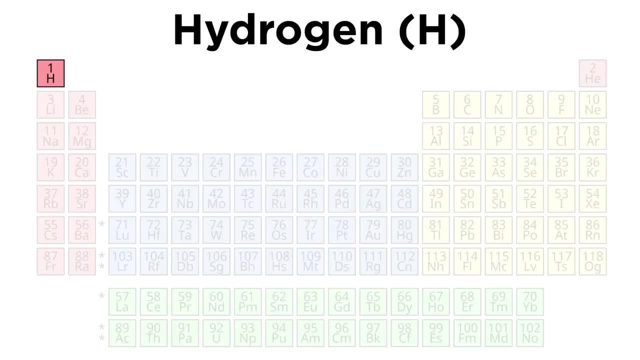 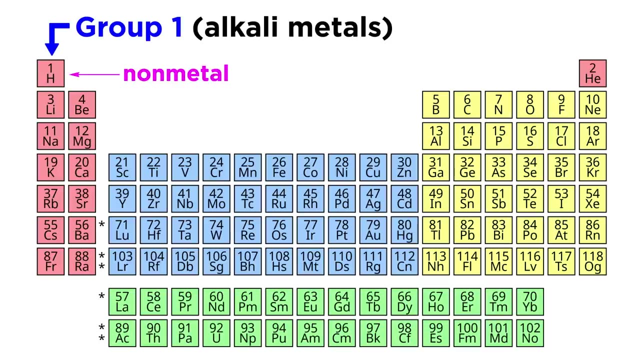 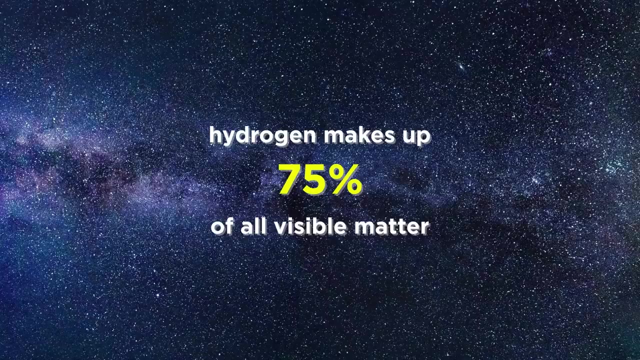 own, as it somewhat defies the organization of the periodic table. It is technically a group one element, but group one is the alkali metals and hydrogen is a nonmetal, And since hydrogen makes up around 75% of the visible matter in the universe, it is ubiquitous in astronomy as well. 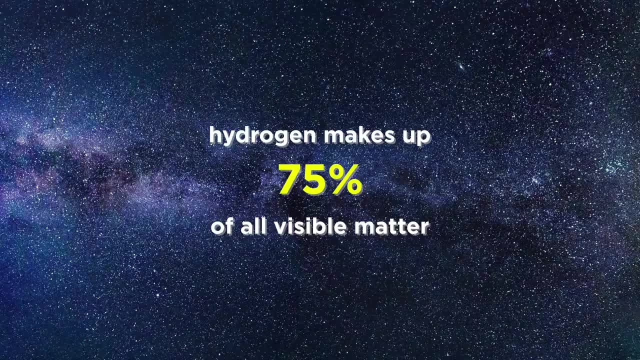 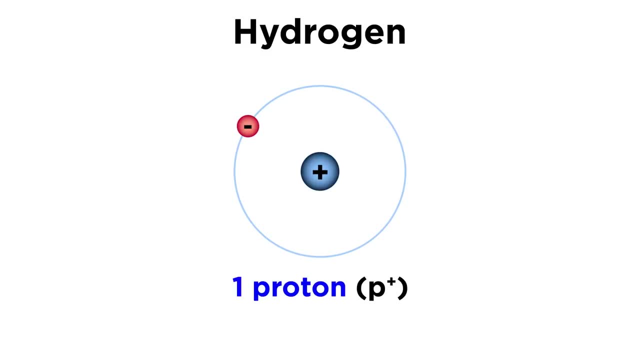 as chemistry and deserves a few minutes all to itself. Hydrogen is the smallest and simplest of all the elements. It houses a single proton in its nucleus and therefore, when neutral, possesses only one electron. In this ground state, its electron configuration is 1s1,. 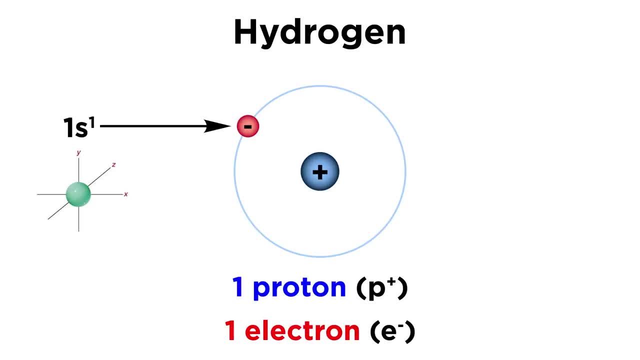 meaning its lone electron resides in the 1s orbital, which is a spherical orbital. There are two other common oxidation states. The first would be plus one which has an electron configuration of 1s0, meaning an empty outermost shell, or simply no electrons at all, which is why 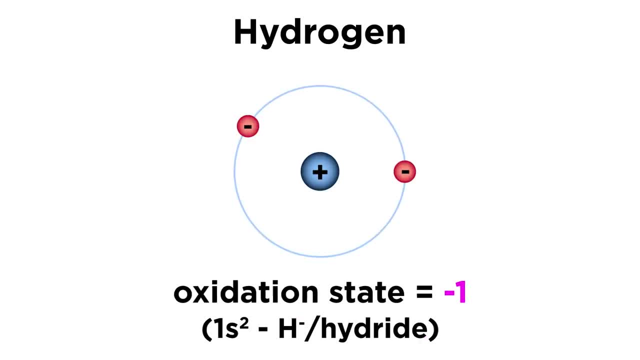 we often refer to H plus as simply a proton. The second would be minus one, resulting in H minus, or a hydride ion which has an electron configuration of 1s2, or two electrons in the 1s orbital. This means a full electron configuration of 1s2.. And finally, the two electrons in the 1s. 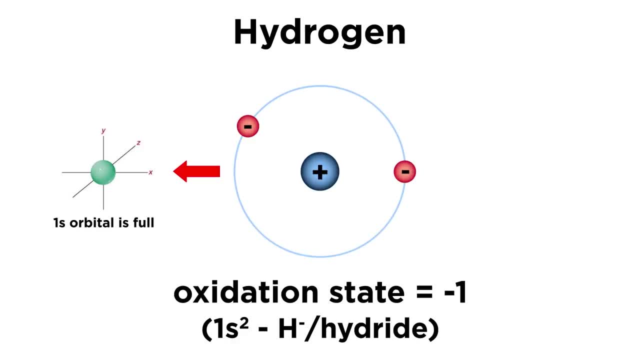 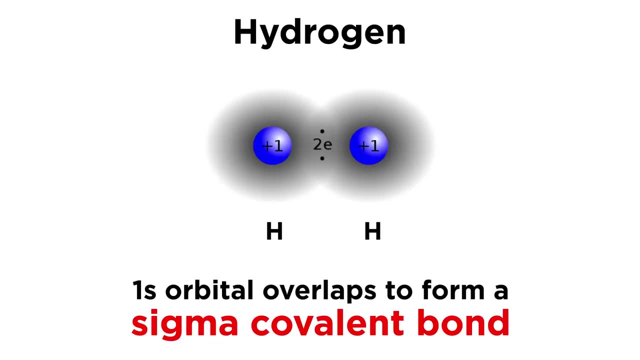 outermost shell, since the first energy level includes only this single s-orbital. Neutral hydrogen with an oxidation state of zero is capable of making a single covalent bond, which involves the overlap of the one s-orbital with some other orbital to produce 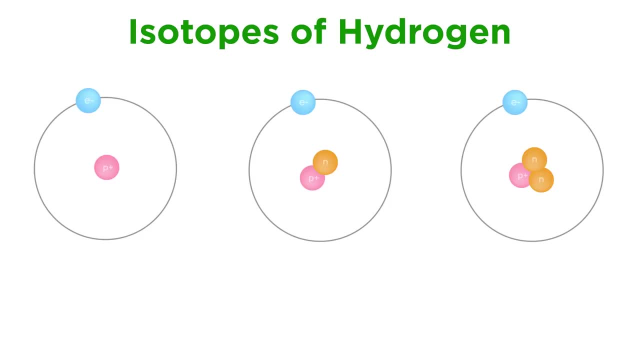 a sigma bond which can occur in any direction. Additionally, hydrogen has three naturally occurring isotopes. One H is called protium, containing just the one proton and no neutrons. Two H is called deuterium, containing one neutron. Three H is called tritium, containing two neutrons. 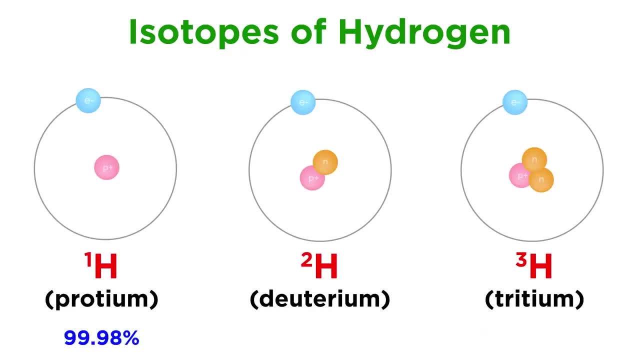 Protium is by far the most abundant isotope, at 99.98% abundance. This is followed by deuterium at 0.0156%, which has application as a moderator in nuclear reactors and is also frequently utilized for isotopic labeling experiments in chemistry. 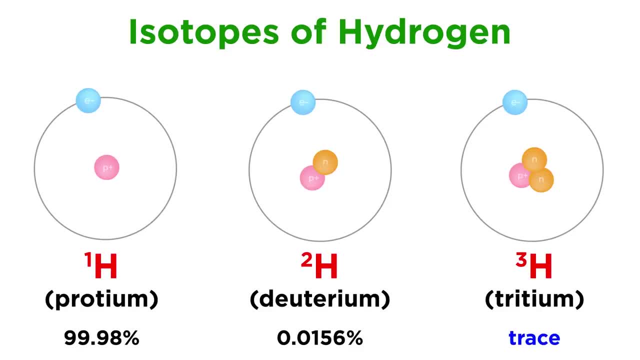 Finally, we have only two neutrons. They trace amounts of tritium, which is radioactive, decaying via beta emission, with a half-life of 12.4 years. It is formed in the upper atmosphere due to collisions between atmospheric particles and 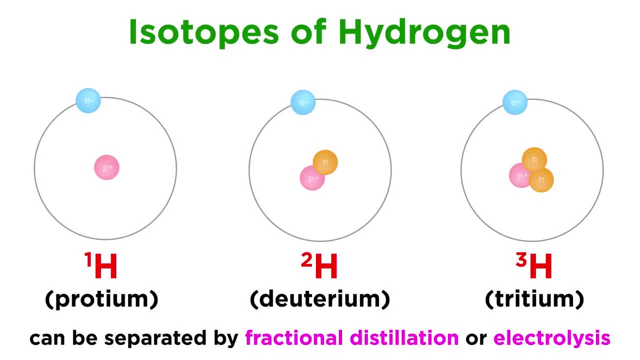 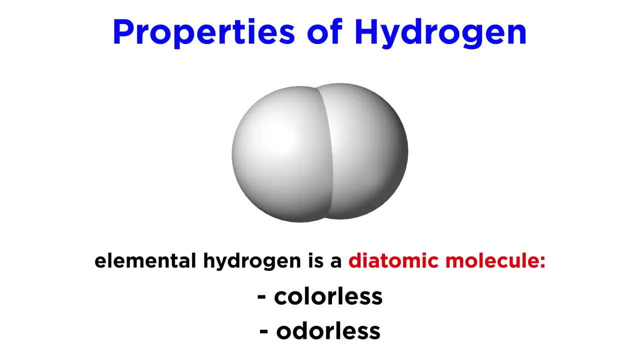 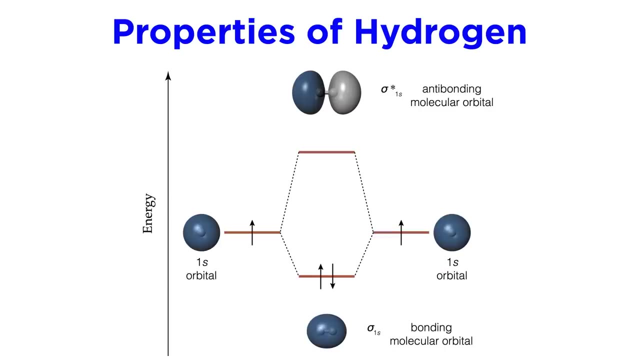 cosmic rays. These isotopes can be separated by fractional distillation or electrolysis, Given that hydrogen atoms can make one covalent bond, hydrogen is diatomic. in its elemental form, H2 is a colorless, odorless gas, And we can describe its bonding behavior with this molecular orbital diagram: 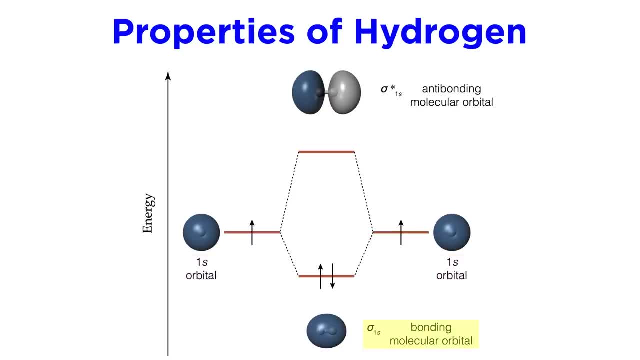 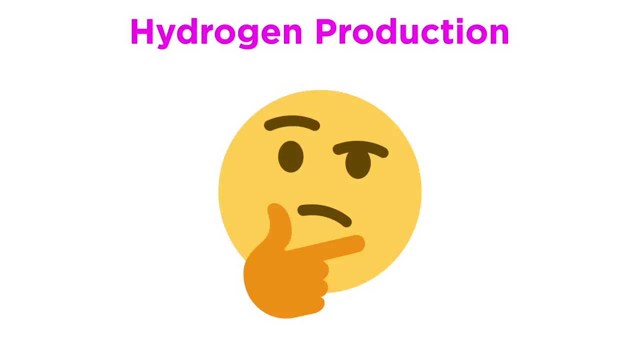 The two 1s atomic orbitals will combine to form a sigma bonding orbital as well as a sigma antibonding orbital, and the two electrons will reside in the bonding orbital, producing the single covalent bond between the atoms. So how do we make hydrogen gas? 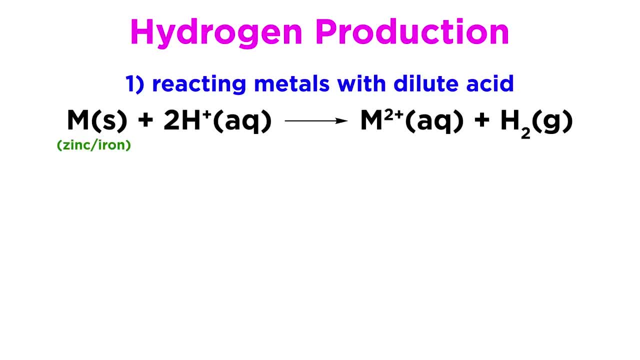 One method is by reacting metals like zinc and iron with dilute acid. The metal atoms are oxidized. The metal atoms are oxidized, Electrons are transferred to the protons and these combine to form diatomic hydrogen. Another method is by the steam reforming of methane with nickel catalyst. 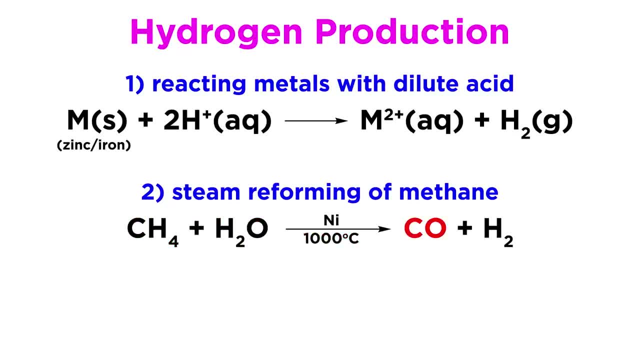 Methane and water are heated to a thousand degrees Celsius, which produces carbon monoxide and hydrogen gas. Finally, there is the water-gas shift reaction, where carbon monoxide and water react over iron and copper catalysts to produce carbon dioxide and hydrogen gas. 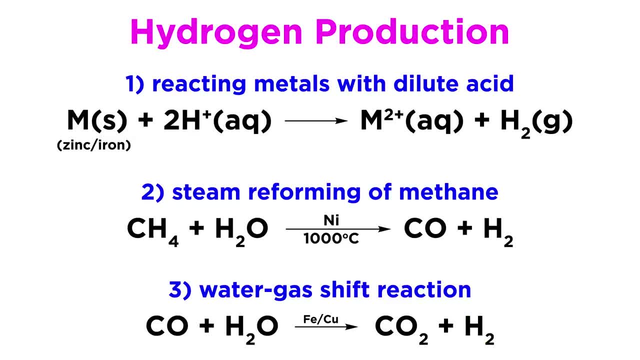 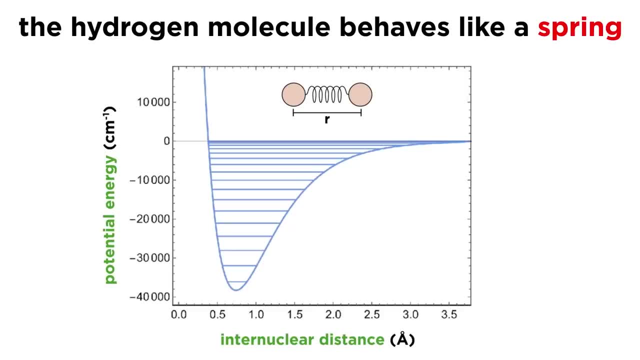 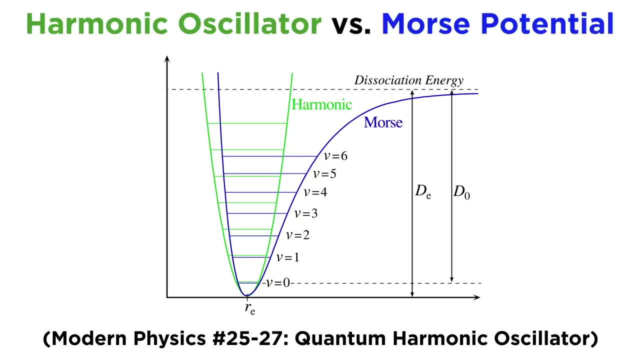 We will learn more about this type of transition metal catalysis later in the series. To look more closely at the hydrogen molecule, the single covalent bond allows diatomic hydrogen to act approximately like a spring. We actually discussed this in some detail when learning about the quantum harmonic oscillator. 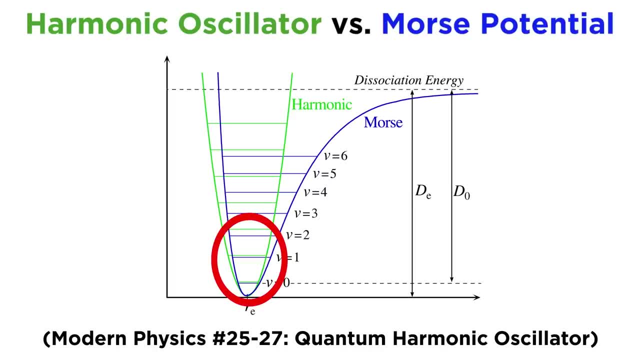 over in the Modern Physics series. When discussing this topic, we talked about how the Morse potential for a diatomic bond is not a single covalent bond. It is a single covalent bond. The covalent bond is an atomic molecule that is approximated by the quantum harmonic oscillator. 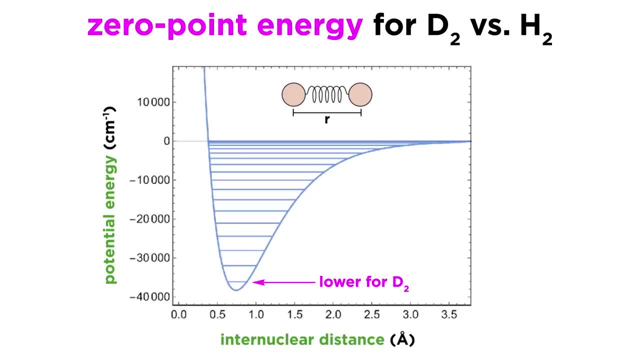 at low energies. To elaborate in the context of diatomic hydrogen, it is the case that when comprised of two deuterium nuclides, it will have a lower zero-point energy than when comprised of protium or a smaller distance from this ground state to the bottom of the well. 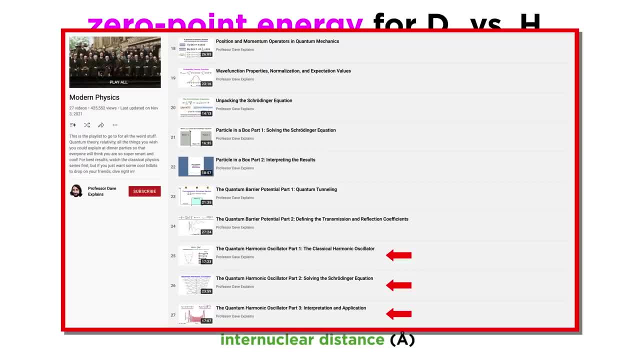 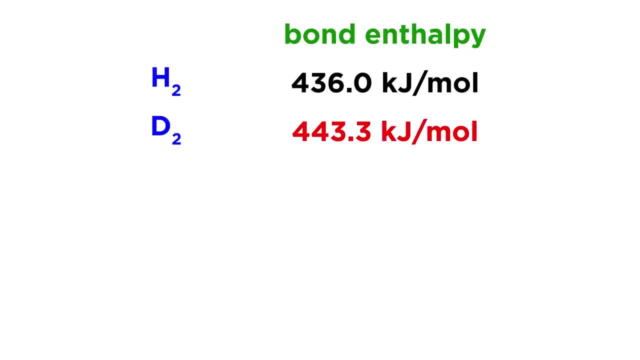 Be sure to visit these quantum mechanics tutorials for more information about what this means and its derivation. Thermodynamically speaking, D-2 has a greater bond enthalpy than H-2, just as D-2O or heavy water has a greater bond enthalpy than H-2O and even a higher boiling point as a more 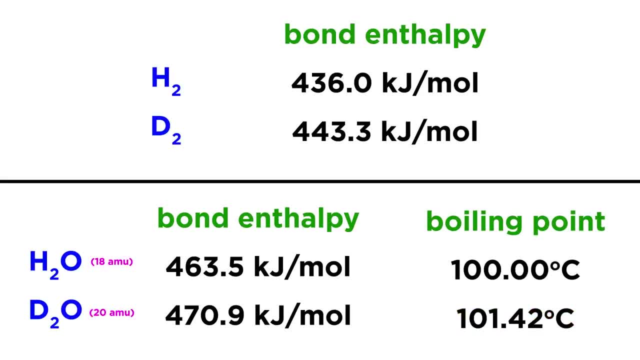 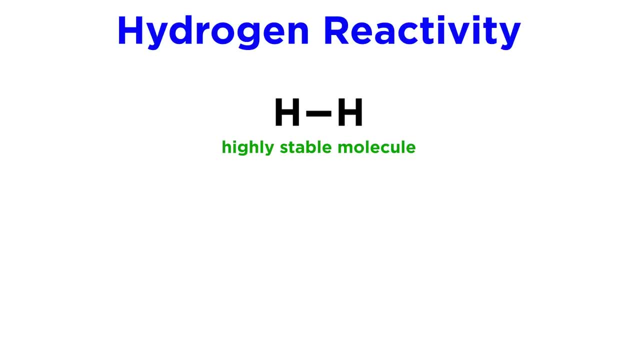 massive molecule will require additional kinetic energy to be liberated into the gas phase. Moving on to reactivity, H-2 is quite stable. We can see this by looking at the activation energy for hemolysis, which will be equivalent equivalent to its bond enthalpy. 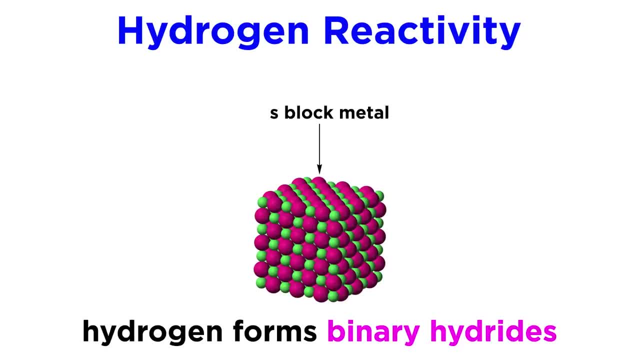 Hydrogen will frequently form binary hydrides with S-block metals. These are non-volatile and crystalline, taking on the form MH or MH2, depending on the oxidation state of the metal. The evidence for their formation is that they conduct electricity when molten, releasing 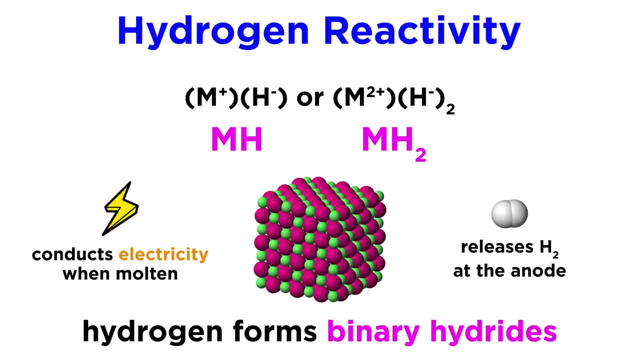 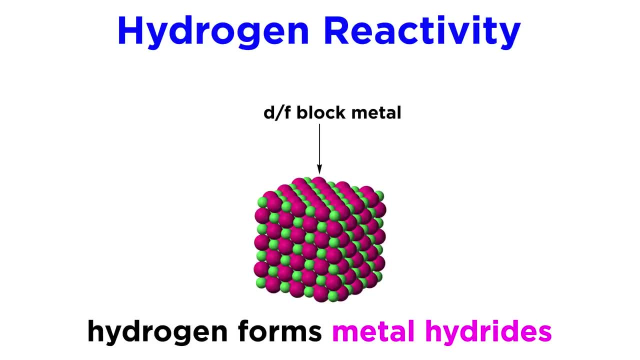 hydrogen gas at the anode or oxidizing electrode. Hydrogen will also form metal hydrides with D-block and F-block metals. First there are bulk non-stoichiometric hydrides where hydrogen atoms tuck into the metal lattice. 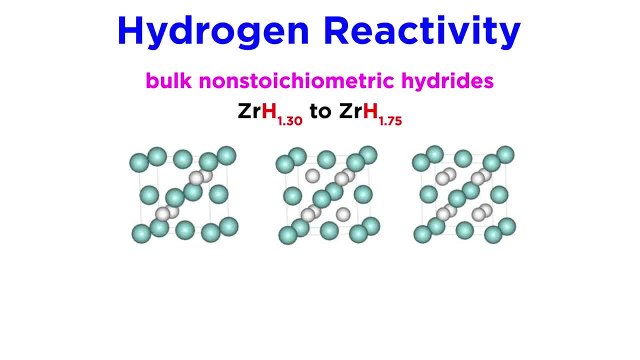 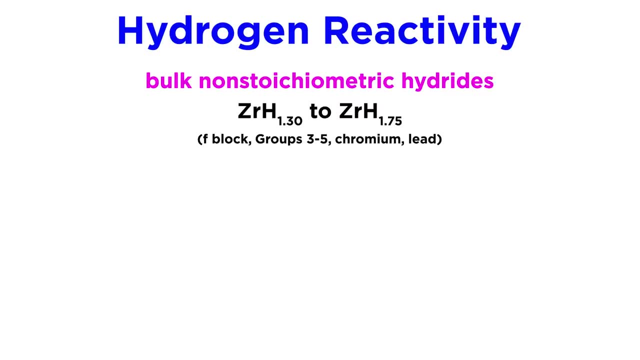 wherever they can fit, sometimes even in non-integer ratios. This works with all F-block metals as well as D-block metals from groups three to five, as well as chromium and lead. Then there are surface hydrides, most commonly seen with group 10 metals like platinum palladium. 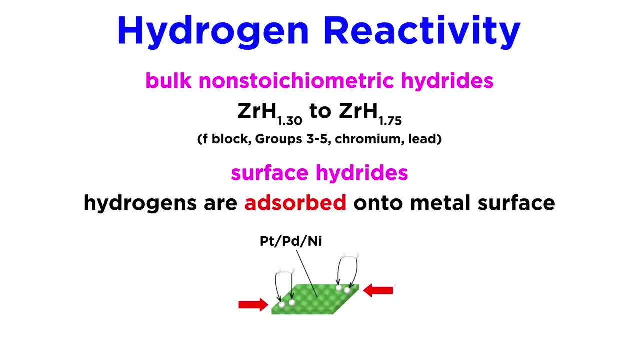 and nickel. Here the hydrogen atoms are adsorbed onto the surface of the metal, activating them for further reaction with organic compounds. This type of chemistry is the basis for much of the catalysis we will discuss later in the series. Then there are also molecular hydrides which are covalent, such as diborane. 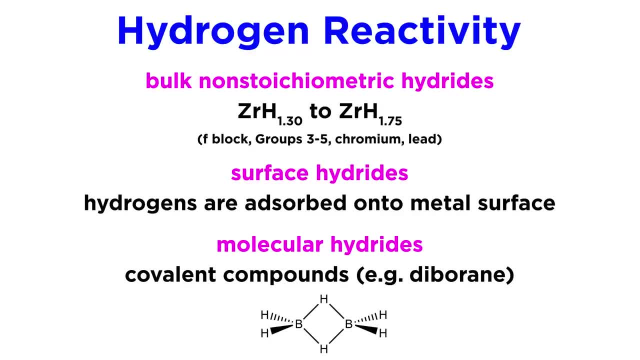 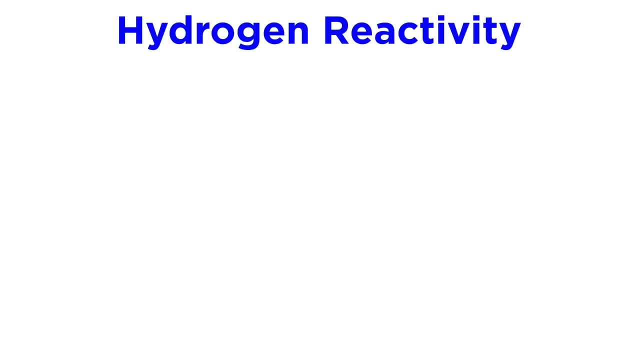 These will be mentioned as we proceed through the table and cover the other elements present in these compounds. Some other key reactivities for molecular hydrides. Some other key reactivities for molecular hydrides. Some other key reactivities for molecular hydrides are as follows: 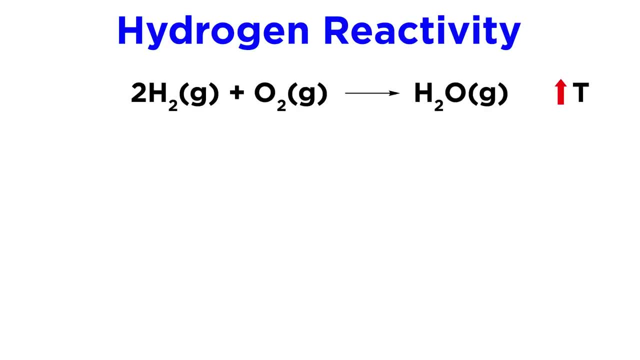 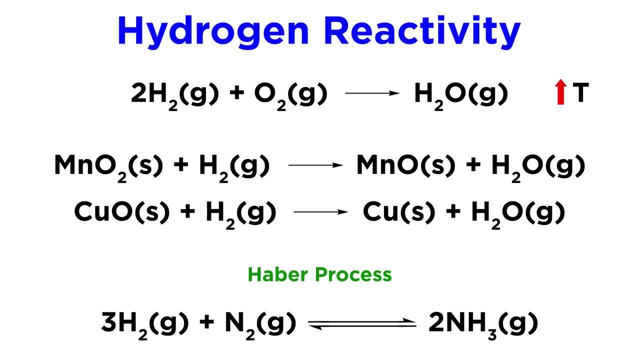 At high temperatures it will react with molecular oxygen to form water quite exothermically. It will react with metal oxides to form lower oxidation state oxides and water, or elemental metals and water. It will react with molecular nitrogen to form ammonia in something called the Haber process. 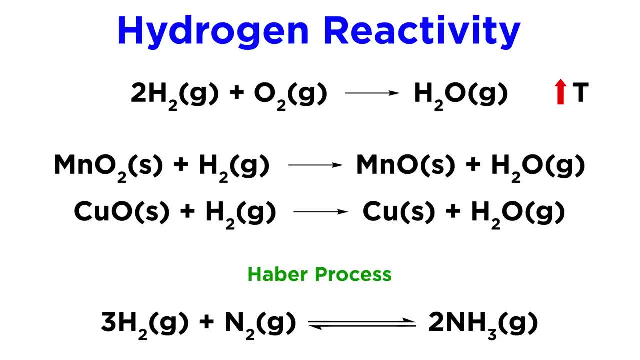 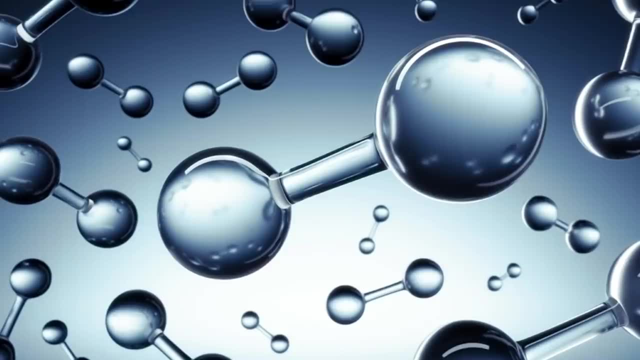 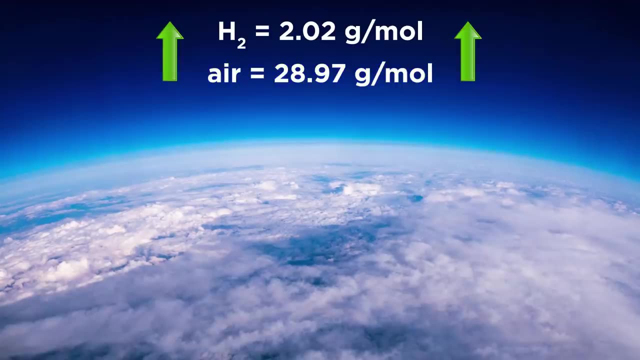 This is a key reaction in the manufacture of fertilizers and it is quite involved, requiring extreme conditions and ferric oxide catalyst. We will discuss this in more depth later in the series. Hydrogen also has a number of other important applications, Given that it is the lightest chemical substance. it is lighter than all other atmospheric components. 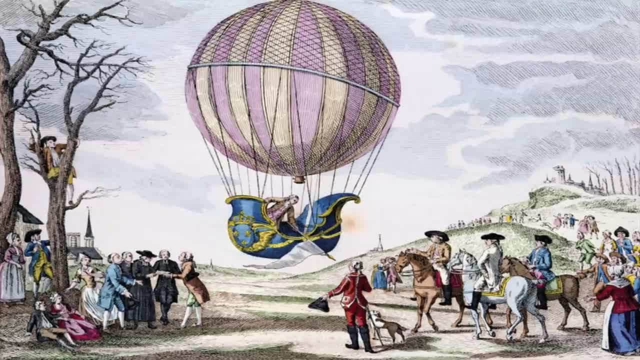 and therefore buoyant in air. For this reason, it was used in early balloons, though it was quickly found to be less than ideal due to its flammability, A lesson that was learned in the early days of nuclear chemistry. Hydrogen also has a number of other important applications. 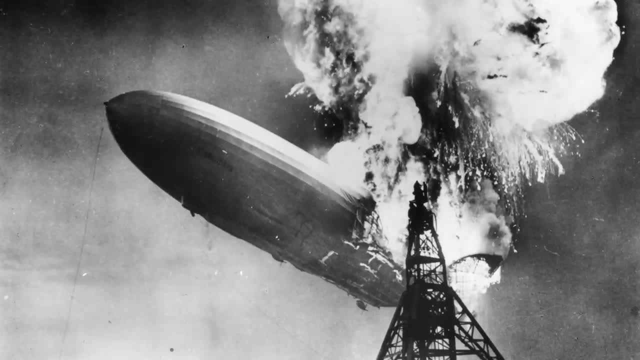 It was used in the early days of nuclear chemistry. Given that it is the lightest chemical substance, it was likely that it would be less than ideal due to its flammability- A lesson that was learned in the early days of nuclear chemistry. 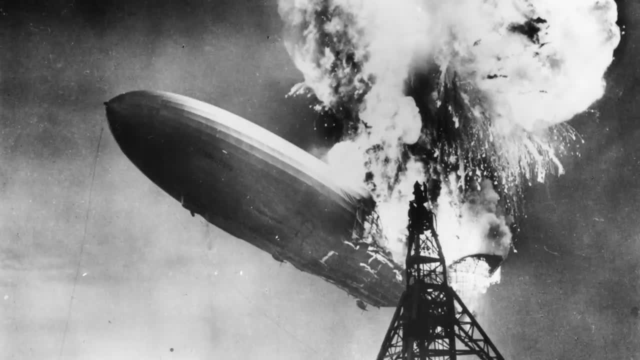 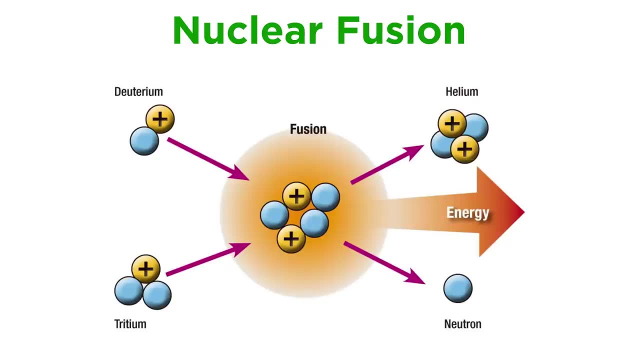 It was also used in the early days of nuclear chemistry. However, in this particular case, the Germans had been using hydrogen, because America would not sell them helium Hydrogen is also used as fuel for nuclear fusion. This is performed inside the Sun and all other stars, where the extreme heat and gravitational 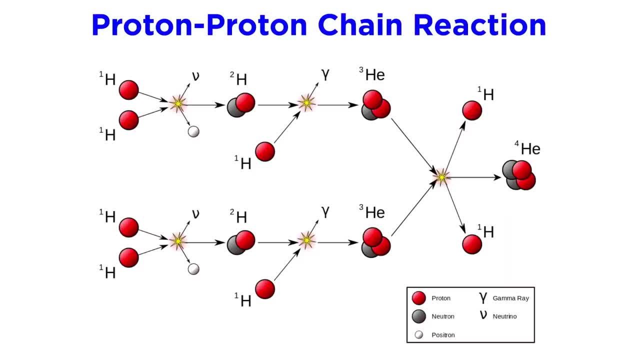 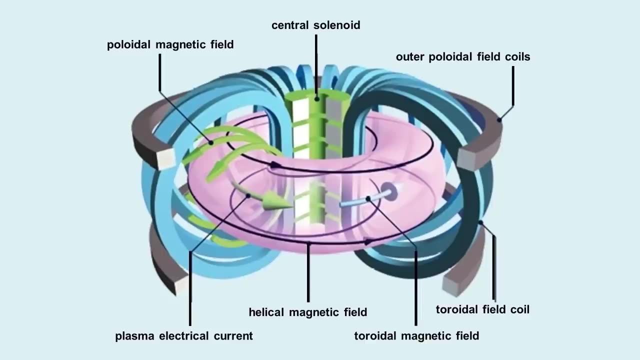 pressure force hydrogen nuclei to overcome the intense electrostatic repulsion and fuse to form helium nuclei is called the proton-proton chain reaction, which occurs over several steps. Here on Earth. we are unable to reproduce these intense conditions inside the sun, so we require 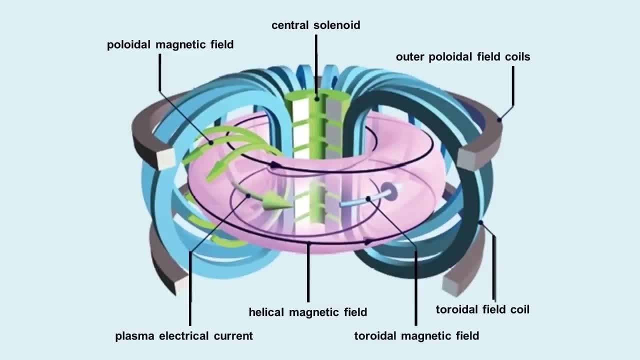 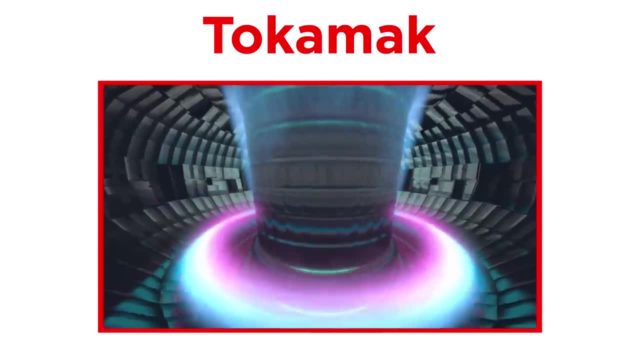 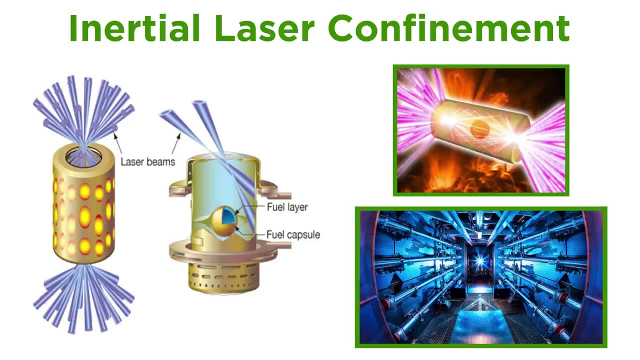 other strategies. We will not discuss them in depth here, but they include electromagnetic confinement involving plasma in a magnetic toroid, such as with the famous tokamak, and inertial laser confinement involving lasers and a pellet of fusion material. These utilize several different fuel cycles which start with collisions between different nuclides.